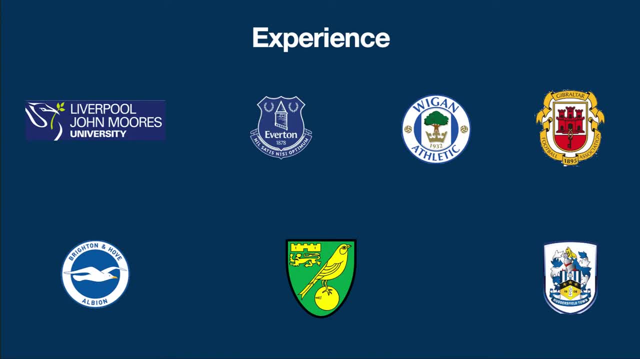 as much as i can. so just in terms of the experience, again, i'm not a person that like speaking about myself, but i thought it'd be good to share where my sort of journey started and where it's gone. um. so i started off studying at liverpool john moore's university. i was doing a course in science and football. 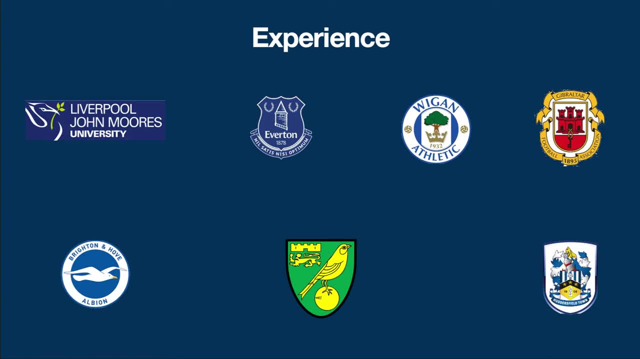 which was really, really good. then i did a master's in sports psychology, got an internship at everton doing performance analysis and sports science with the first human academy. i then went on to coach at wigan athletic academy- uh, with the under under tens at the time. 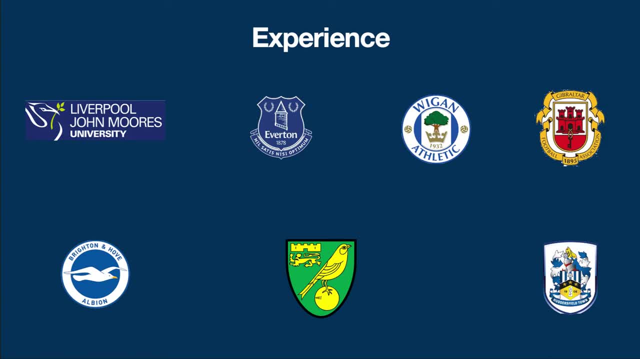 i also did some work with the gibraltar national team, coaching the 17s and the 19s. then i got a full-time internship at brighton and then from there got a full-time role at the club within the first performance analysis department, went on to move on to norwich as the opposition. 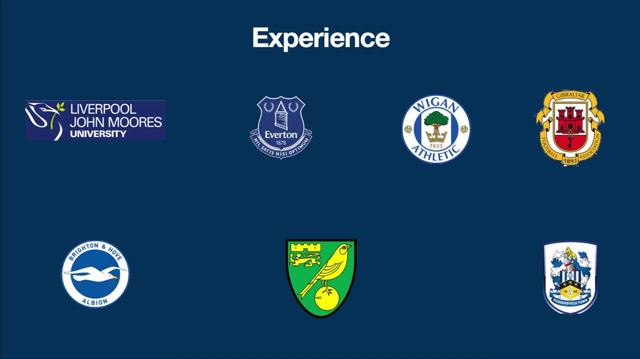 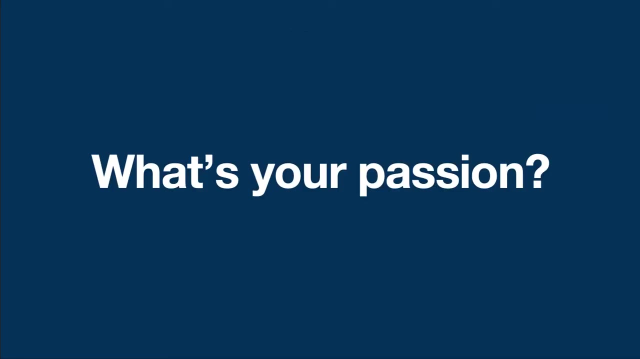 analyst for two seasons and then went to huddersfield as the opposition analyst and eventually got promoted to the head of analysis. so i was there for nearly four years. so yeah, that's just a bit of experience in terms of my background. it's really important that you understand before. 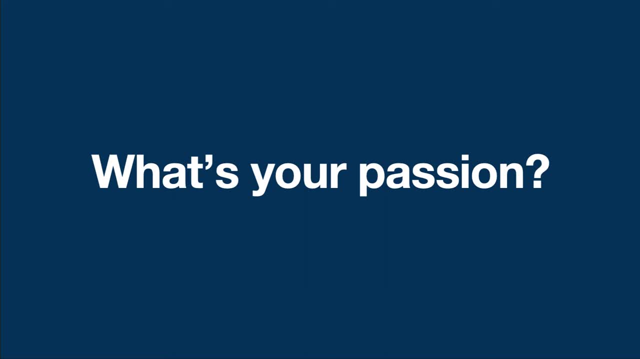 you go into anything that you know, you try and find what your passion exactly is, uh, what is it you enjoy doing? what is it you really want to do? um, in terms of a career, in terms of a, a job? um, because once you do find that out, we have a good idea of that is then it's uh. 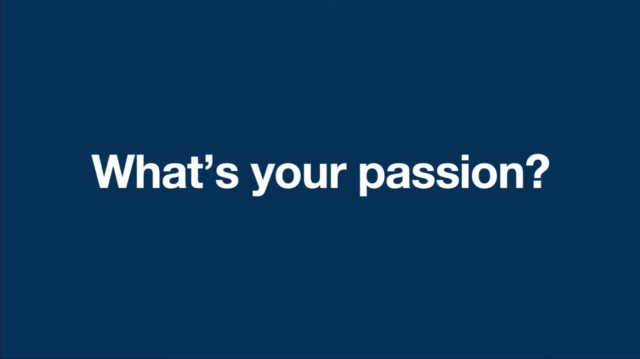 you know, you world your oyster. there's no limits in terms of where you can go. but first of all, the most important thing for me is to find out what you really love, what you enjoy, what are you passionate about, and then and then take it from there. so, whether it be an 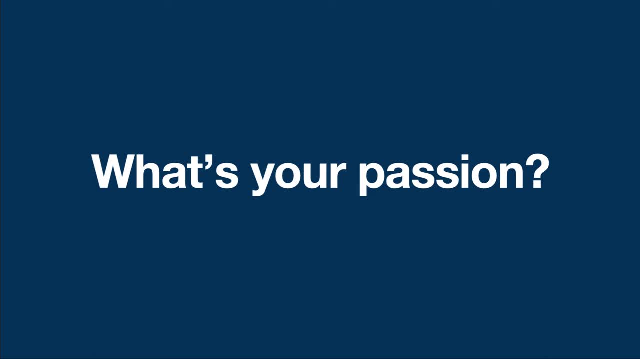 whether it be coaching, whether it be fitness coaching, whether it be physiotherapy, try and find what it is um and then go for it, and then just just give everything you can to that. so, in terms of the performance analysis, um what the main duties, roles and realities are, 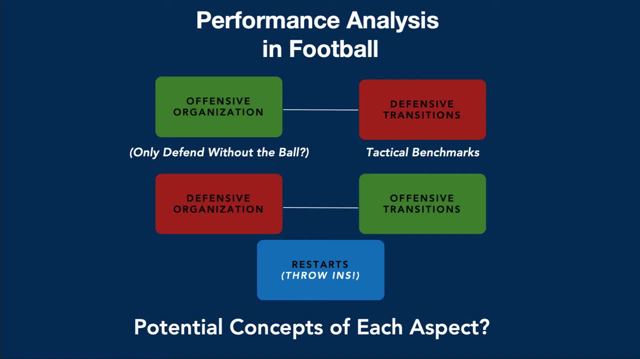 off the roll. so, before we start, just a quick overview in terms of how we broke down performance analysis and football, how we looked at the game tactically, because there was a lot of involvement in terms of tactics and game plan. um, so we divided into, obviously, the four parts of five. 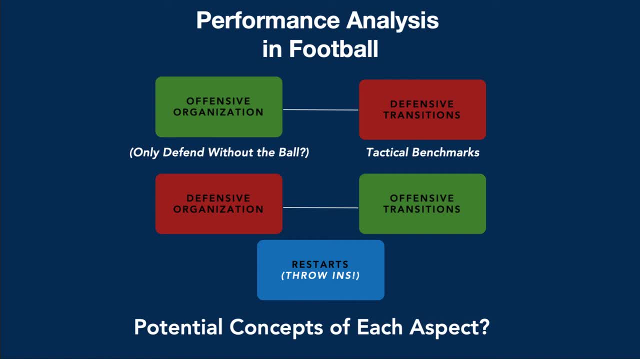 parts, sorry: offensive organization, defensive transitions, a defensive organization to offensive transitions, and then restarts, which is obviously uh when the ball's out of play. so throwing goal kicks um corner free kicks, um highlighting throw-ins there, which is a really important aspect in the game that doesn't get looked at enough, in my opinion. uh and um. 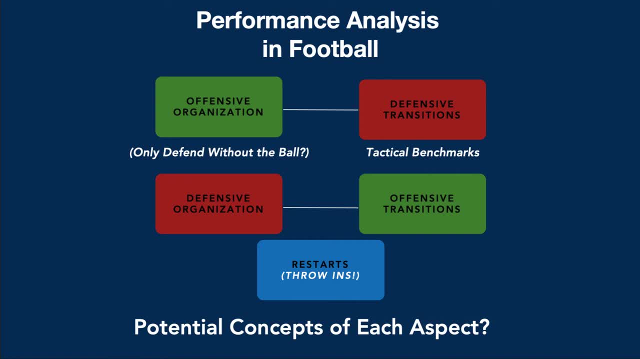 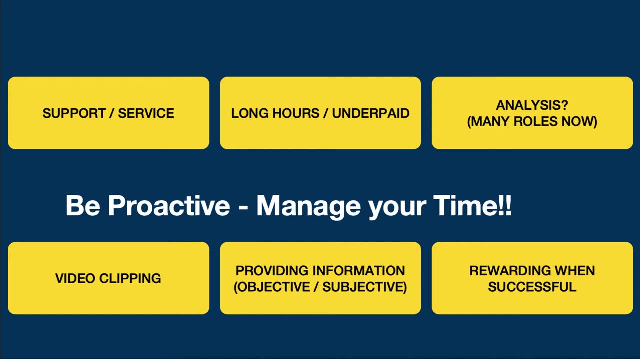 um, yeah, those are so how we sort of analyze the game. so, in terms of the actual role, uh, main duties, um, and realities of it, you realize is it's it's long hours, it's normally underpaid, so just to put that on your radar, listen, you will get some roles that. 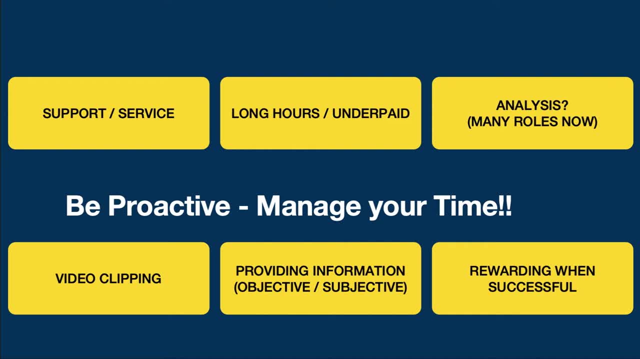 are well paid, but you've got to sort of work for that and work your way up, and at the beginning you probably have to do a lot of internship, volunteer work. that's just part and parcel of the career. um, um, but that is a reality, uh, unless you're very lucky. 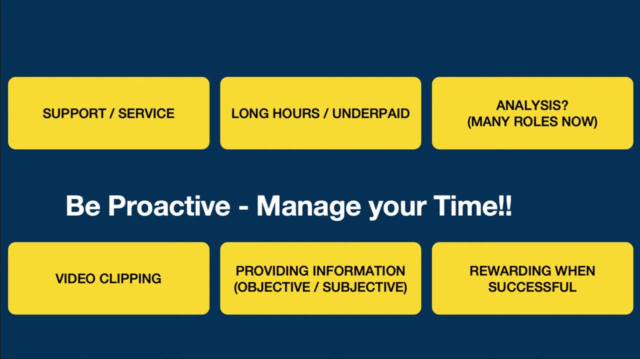 um, support service. you're there to support the coaching staff, the players. it's a service you're giving to the, to them and to the club. um, there's a lot of roles now with an analysis, so it's all. uh, you get things like now like individual analyzed. you get opposition analyst you. 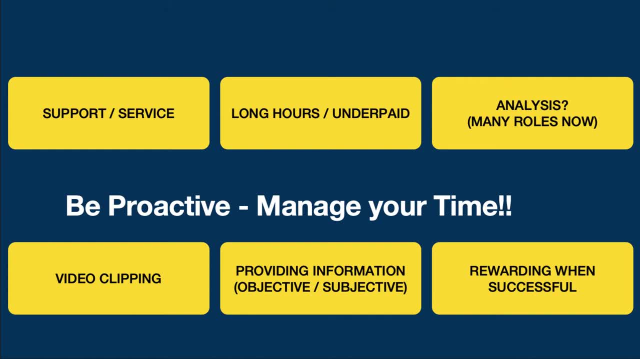 get a post merch analyst. you get to set plays on a list. you get um goalkeeper analyst. you get so many different types of roles. now also get recruitment analysts who are involved in the scouting side. so there's so many more roles. it's more broader now. you will do a lot of video clipping with programs such as sport code. you know. 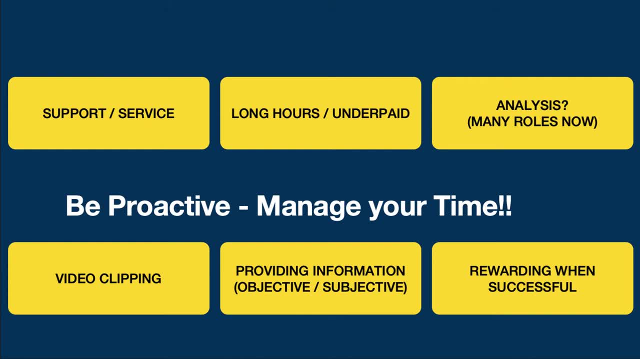 them type of programs where you clip a lot of video when you're watching games using the cold window. you're providing information be objective and subjective, so some of it can be objective in terms of the data which is growing a lot now in the in the area of performance analysis and 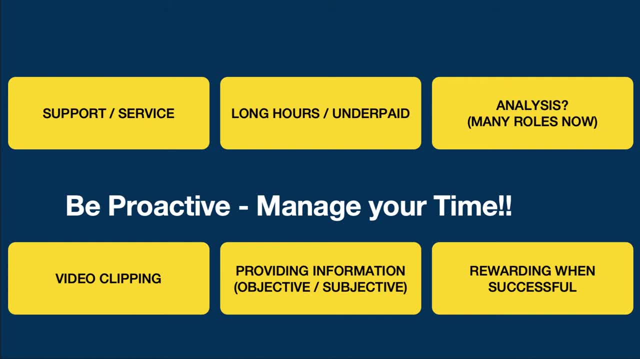 obviously a lot of it can be subjective, can be your opinion when you're watching a game. you might have a particular opinion on an instance in a game. that can be very subjective and it can be rewarding when you're successful. if you do the well, there are benefits and there are strong rewards to the 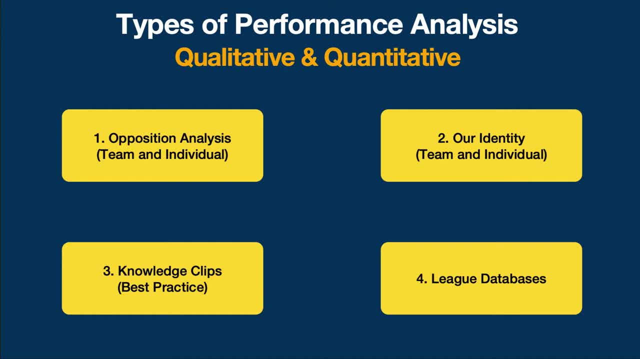 job. so what are the different types of performance analysis? obviously you've got qualitative analysis and quantitative analysis. like i said before, qualitative analysis could be video- yeah, it's more subjective, it's more opinion based, uh- whereas quantitative it's sort of objective of information, such as statistics, um. so those are the differences which which which you both use. 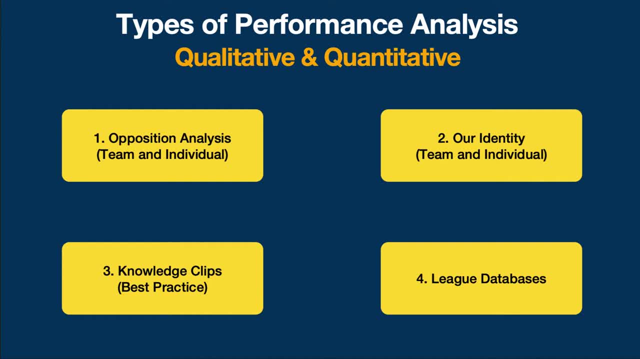 uh, which, you sorry, both are used within, within performance analysis, so different four part of the four different parts that we probably say we use, um, it's opposition analysis, both team and individual, the identity of the particular team. so, individually and collectively, uh, how do they want to play? uh, what is the style, what the training methods, what? 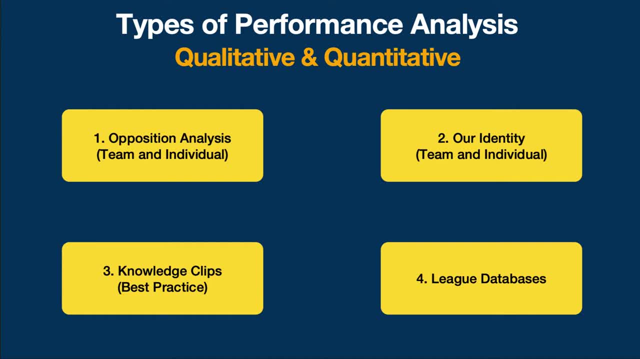 is the sort of methodology of the club knowledge clips which are best practice. so watching teams like around adrid, barca, liverpool, man city, these type of teams where you're getting the best, best clips, benchmark clips to to work off as ideas and as examples, and then you have a thing. 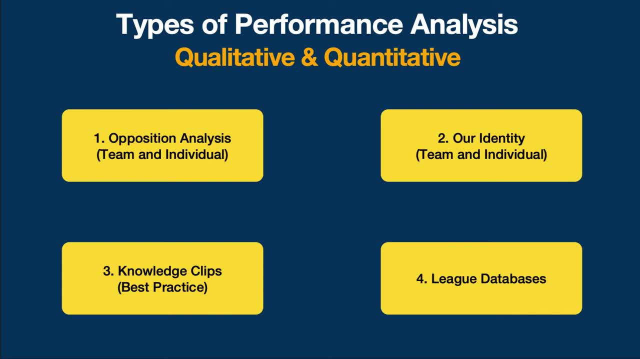 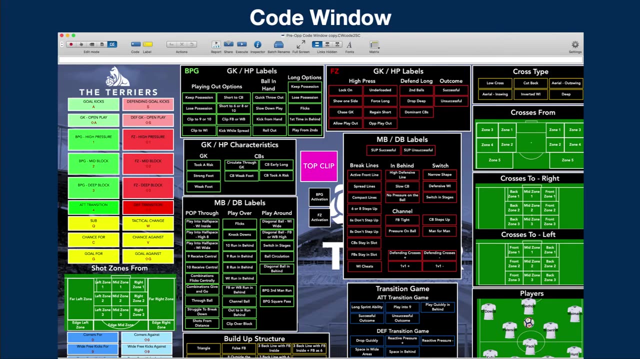 with the league databases, so we had a database for all the set plays, all the chances on the goals within the championship, um as a database, which was really good information both for qualitative and for quantitative analysis. so the code window is really important, um, it's going to be a very important part of your, of your working process when you do get into a performance. 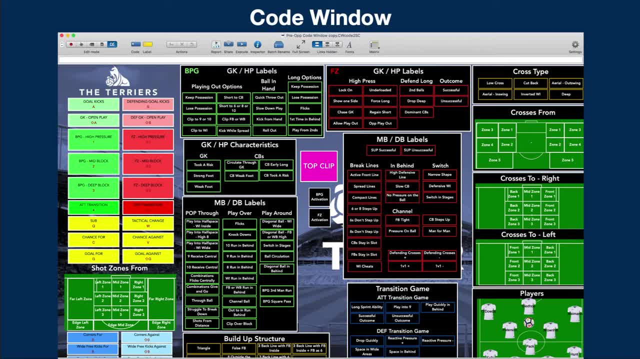 analysis. obviously this one looks a bit complicated, but, um, you know, essentially you've got the codes, you've got the labels describe the codes, and then you've got the, the, the notes, which act as an extra layer of information so you can create your own code window. you know, you can make it very, very. 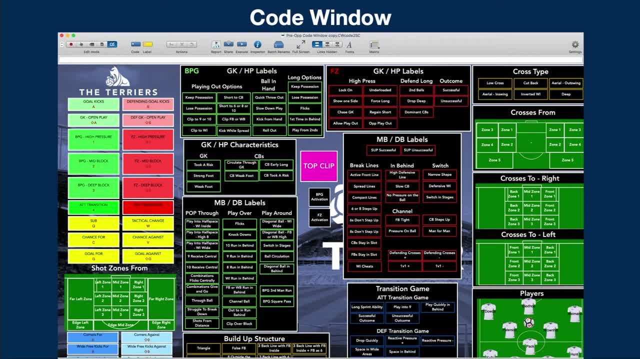 you know, you can add some different colors once you get to know how to use the software. this is a sports code example, but there's so many things you can code and you can get stats and information for- uh, you can be quite creative with it, which is really good. so that's just an example of one. 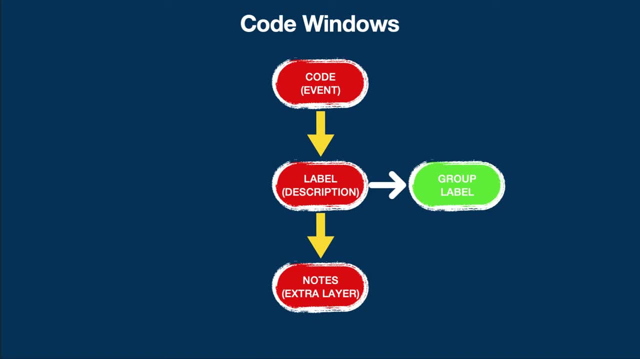 that we use. uh, like i said, essentially it's the code which is the event. maybe it'd be a goal kick, for example, uh, and then the label describes the event, and then the group label uh would be the sort of grouping of that particular label, um, and then you've got the notes, which become an extra. 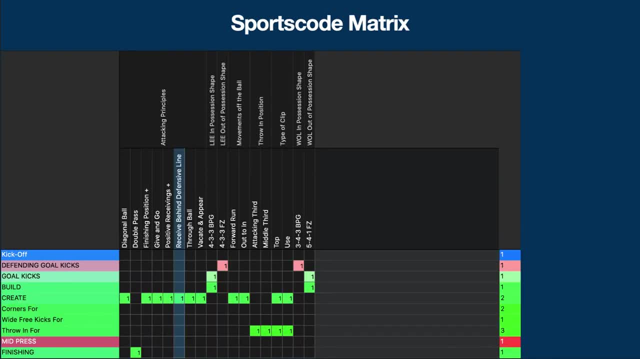 layer. so this could be a practical example. so this is the matrix in sports code. so you've got um, the defending, cold kicks, goal kicks, build, create, so they're sort of the events that i said. they're the codes and then obviously you've got the group labels on the on um, on the right side at the top. 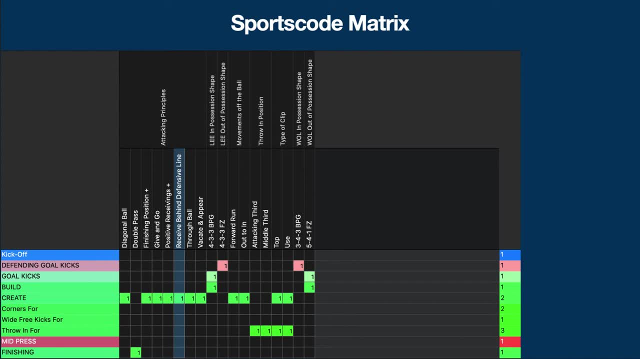 attacking principles. uh, movements off the ball. so the group label is the attacking principle and then obviously them, their them labels are the ones within the group of attacking principles. so then you've got diagonal ball, diagonal pass, so they're all part of um of the attacking principles and they go under that. 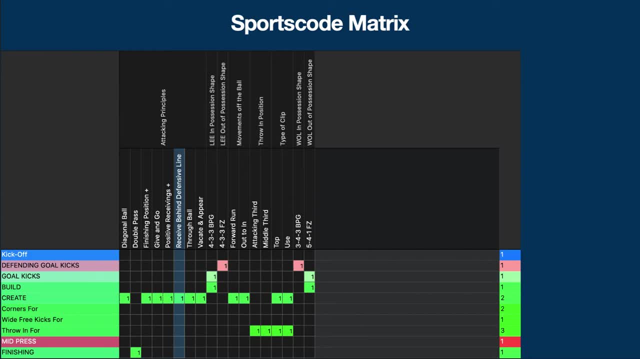 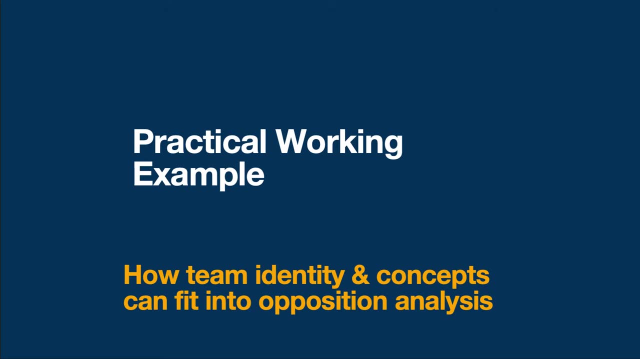 group, uh. so there's obviously an example of what i meant and how it looks like practical working example, uh, so how we can use team identity concepts to fit in opposition analysis. so this is just an example of of work that we did in terms of trying to find clips of best practice to then. 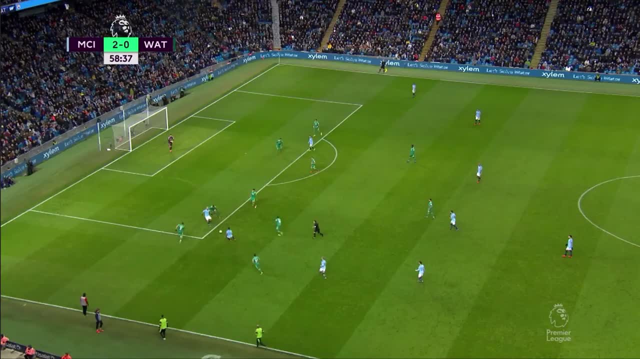 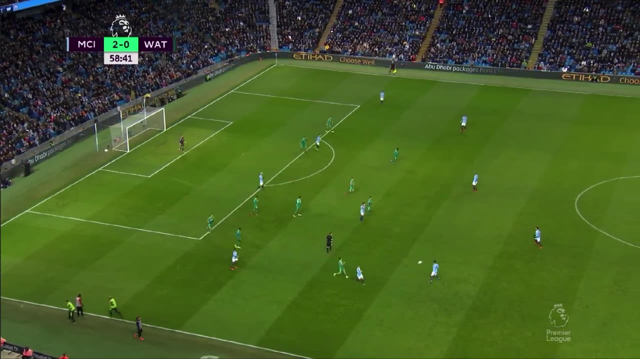 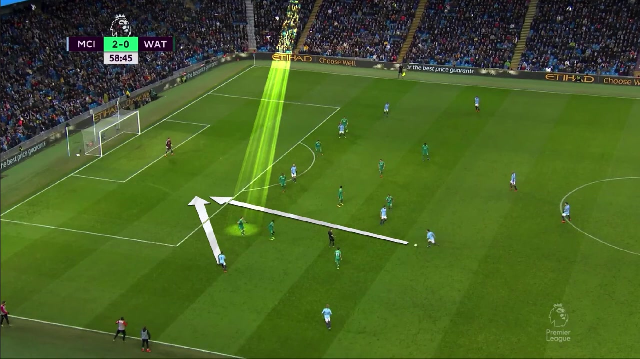 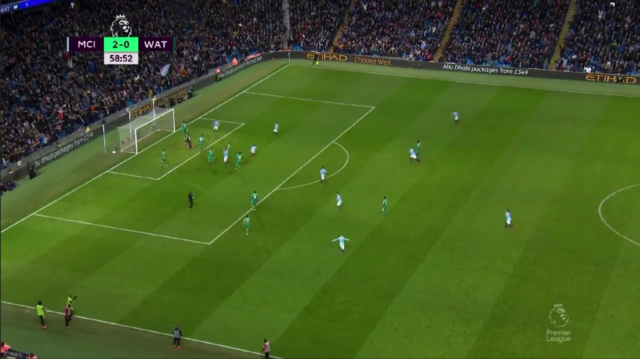 introduce to the team and how they want to play. there's an example of man city. so this is a sort of through ball with an out in run. so it's a. you're breaking the, the line invented the defense, the defensive lines. it's a run, bang through wall in behind the defensive line, cut back inside in a goal. so this is an example of mancity. um, then, just a bit on the analysis process. so, um, we look at the analysis process. so, uh, we look at, Ahhh, Mitra 2, new match forced. look at donate against brother to be offered to targeting the an ultralet 부�mer. a little bit of at least three games a week, then the 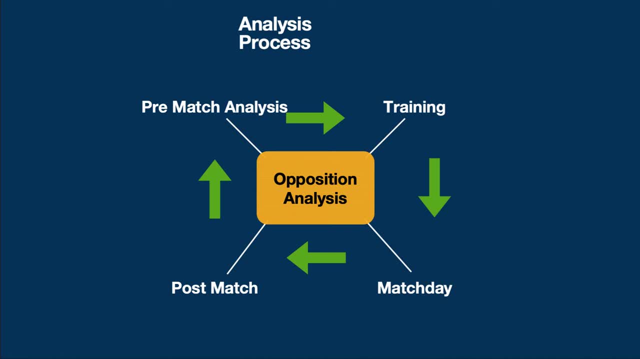 we look at pretty much analysis and the opposition probably watch, you know, depending on the team, maybe four to five games on average, obviously games that would be relative to how we play with teams maybe playing a similar shape, a similar way of playing. so obviously it's relative. 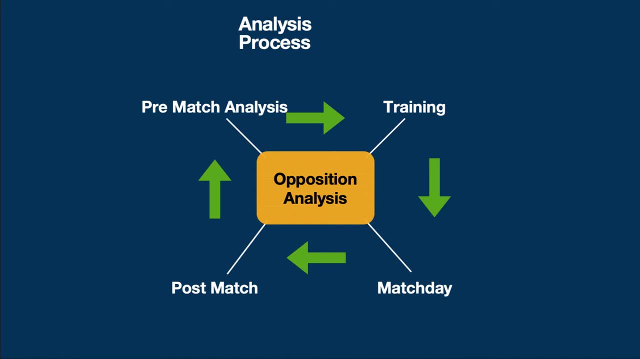 to how we want to do it, so you can get good examples if it works well or bad examples if it doesn't work well, and how that particular team react to them sort of shapes or them styles of play. so once you've done your pre-match analysis, 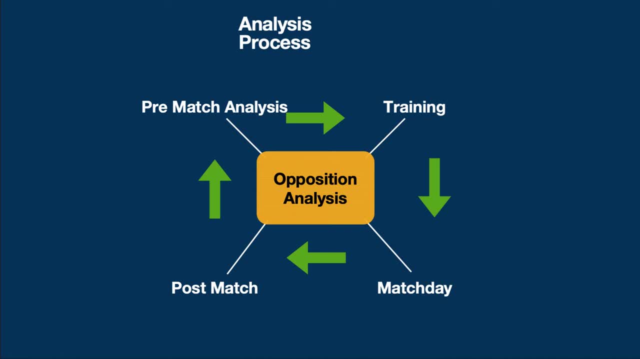 you've had a meeting with the coaching staff, you've identified what the themes are, how the opposition team play and things that you want to work on and you can introduce it in training. obviously then that goes into the match day also, introducing video meetings so the players can see. 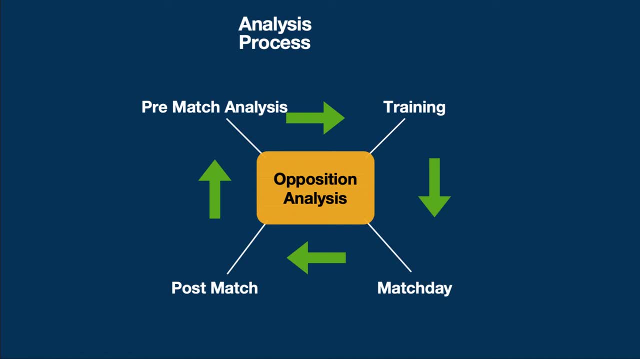 the clips once the match day happens, then that goes into the post-match, once it's finished, and then it's a sort of cycle again: start with the pre-match, start with the next team, the next opposition that we have to play. some advice on networking. it's really important. 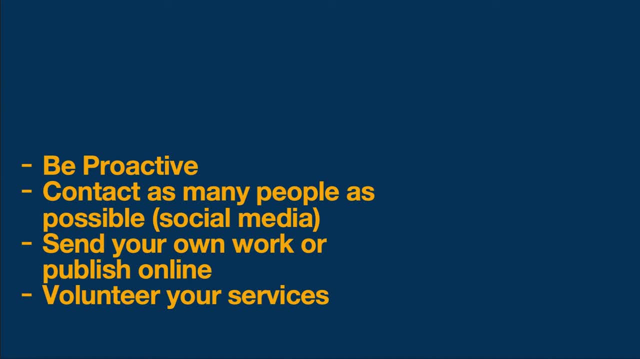 to be proactive. it's really important to be on the front foot to go and search for things. Google try and contact people you know. especially nowadays, with social media, it's a good platform to be able to publish your work online for a lot of people to see. 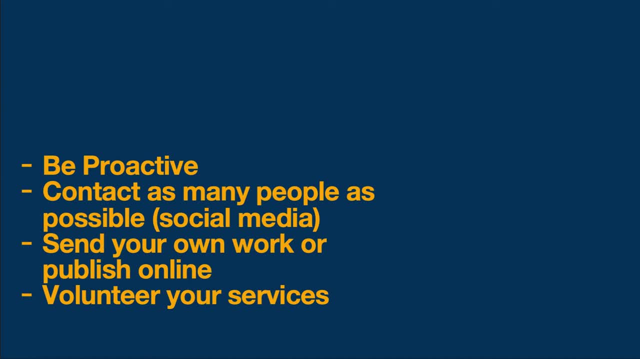 so you can, you can affect a big audience. so it's it's a powerful platform. so try and use that if you can again like be proactive, contact different clubs, contact different people. maybe LinkedIn is another one- find out people's emails, maybe go to the particular club. 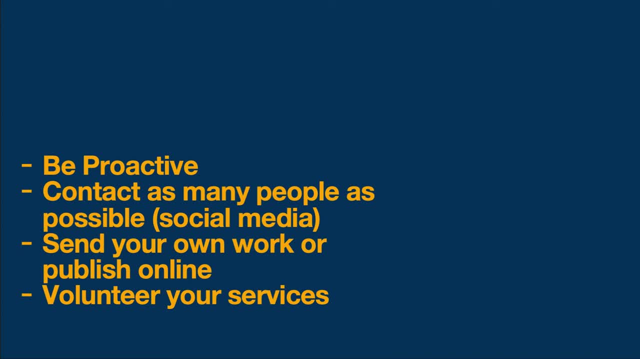 try and speak to someone there, but just be proactive. you know the worst thing they're going to say is no, but at least you know you've tried rather than not trying at all. and you never know, one person might might give you that chance. that's all you need. 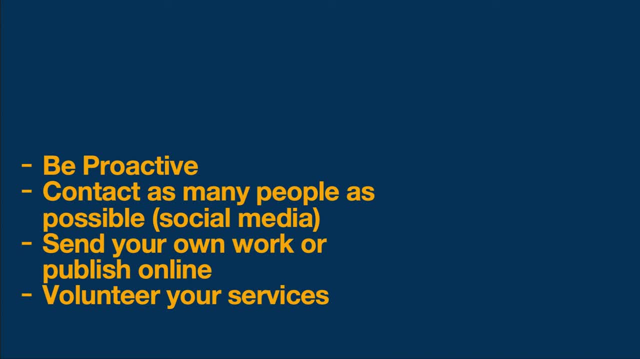 again. send in your work. send your work to people or publish it online so people can see it. try and get feedback for it. volunteer your services. so go and say: look, I work for free. just be proactive, like I said, show people that you really want to do it. 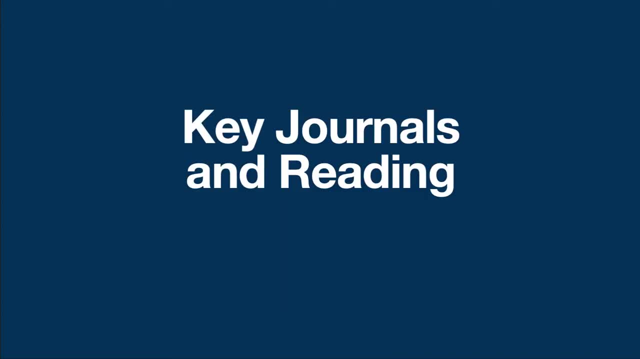 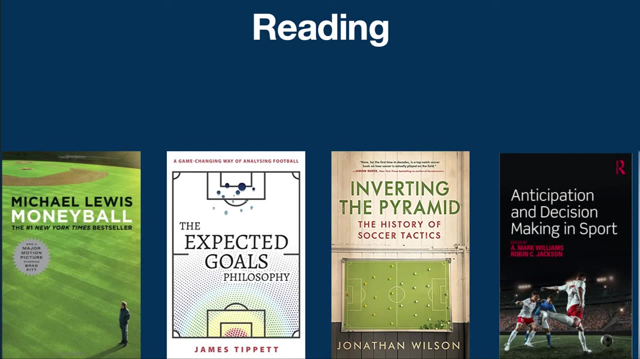 and you want to get involved and you're very interested touching upon key journals and reading, which is really important. so these are just a couple of a couple of books that I've read and I can recommend. so the Moneyball one is quite good in terms of Michael. 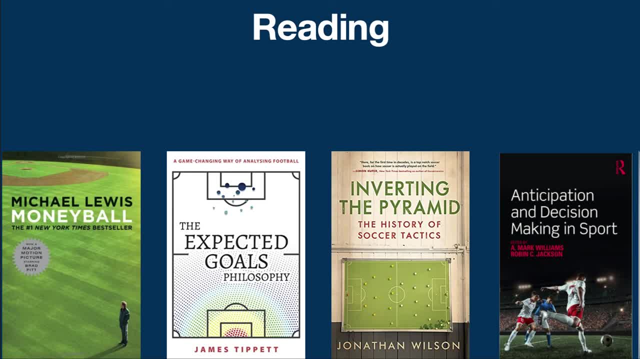 Michael Lewis. obviously I imagine a lot of you would have seen the film. if you haven't seen the film, make sure you watch it. really good film just in terms of how stats and how data analysis can influence a sporting environment. so it was to do with a team in baseball. 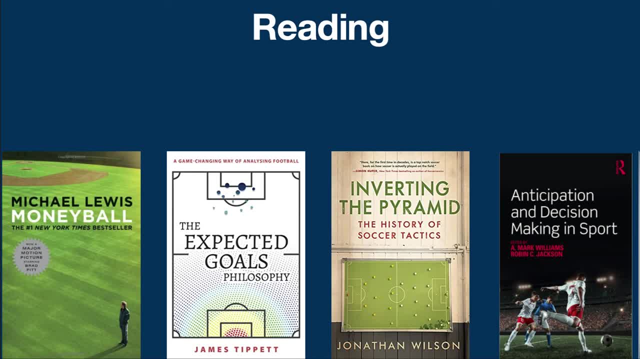 but that can be related to football, that can be transferred in terms of the process, in terms of the principles of it and the importance of using statistical analysis to inform your decisions and to form a working process for the club. obviously it was based more around sort of recruitment and scouting. 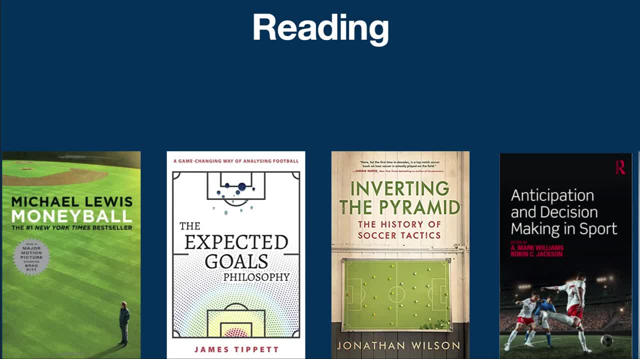 in this particular book, and for me- I can't tell you how much, because I think it's very important to include a kind of personal analysis in the book and then you can then apply that to a team analysis or a position analysis, etc. etc. another book which is important: 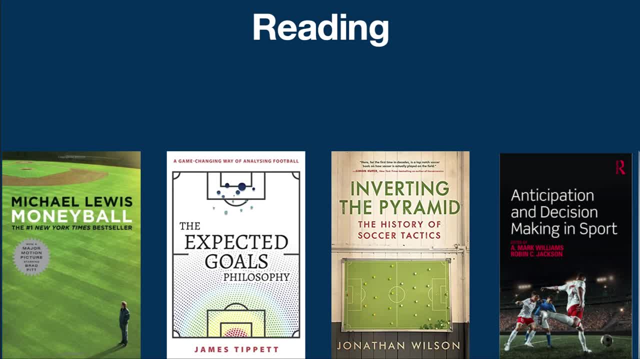 is the expected goals philosophy. I thought it was a really good book. again talking about statistics, in particular, expected goals stats and the importance of it, I think it's a really good book. I think it's very practical how you can apply it to the football world or sporting world. 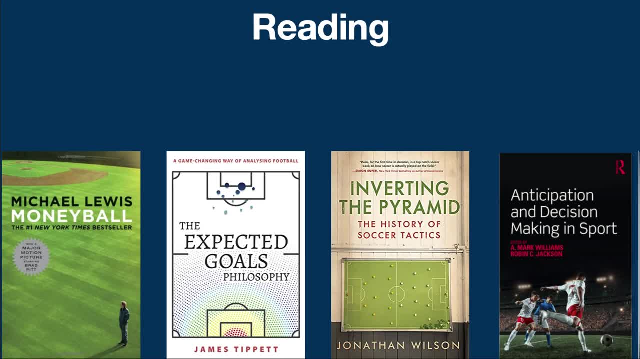 it's a really good point in that book And I think it's definitely the way forward. It's always growing now the data analysis and stats. They're really growing within the industry of football in particular, So I think it's something that's something definitely to take interest in. 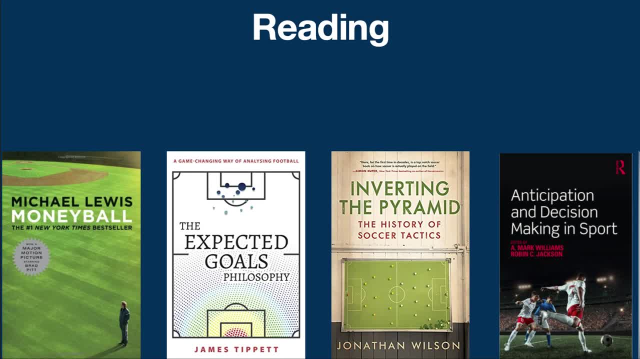 For those tactical geeks- if you want to call it- that really enjoy football tactics, I would recommend the Jonathan Wilson book which is called Inverting the Pyramid. So yeah, essentially it's a history of football tactics from the 1900s, when football began, all the way through to nowadays. 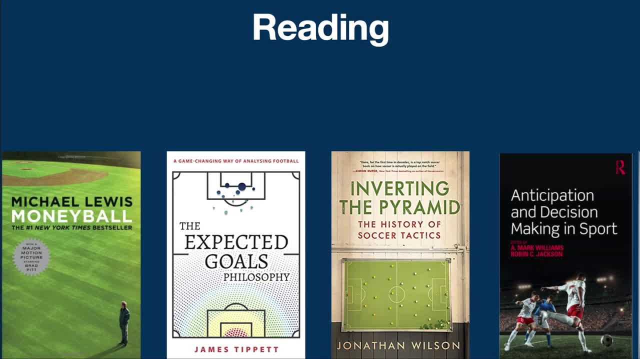 going chronologically throughout the years and how it's developed and how it's changed through different parts of the world. Very interesting book, So I would recommend as well to get an understanding of tactics in football And then the one and more perceptual cognitive skills. 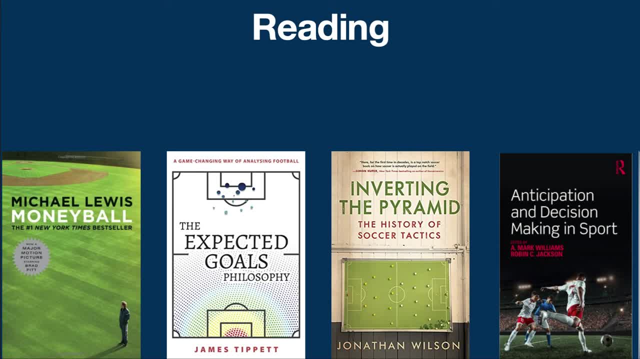 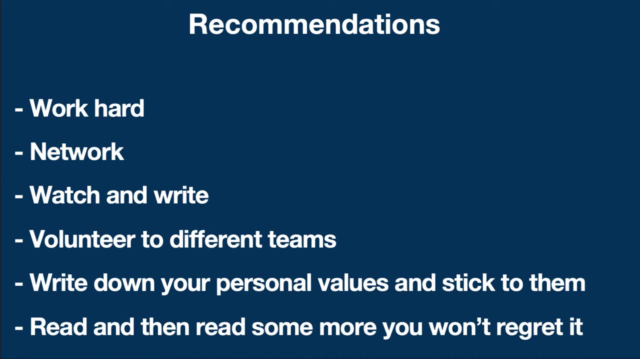 and motor skills and how people learn, and how people learn in sports And the sort of decision making. So again, the perceptual cognitive skills and how they're developed and trained within sport. So interesting. So just to finish off, really, my recommendations would be to work hard as a principal. 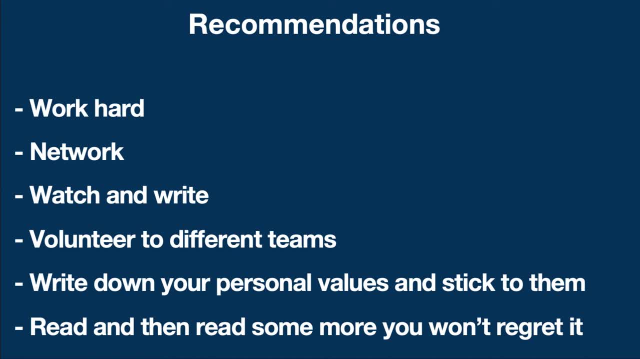 Make sure you work hard on whatever you do. Just give 100% every single day, Try and learn, try and be a better person and a better professional. So, yeah, it's very simple, isn't it? But it's very effective. 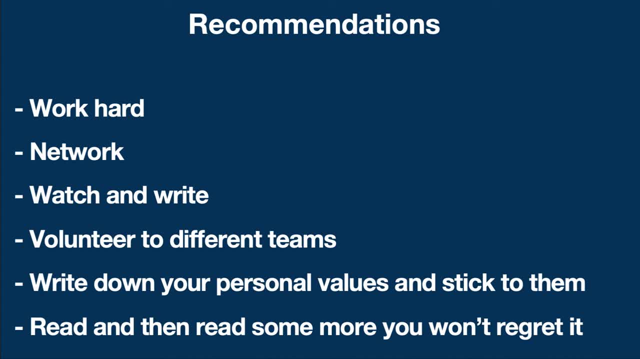 So if you work hard, I believe you always get results and try and work harder than your competitors and other people around you. But again, it comes back to finding your passion And then, once you find your passion, you can dedicate yourself to that. 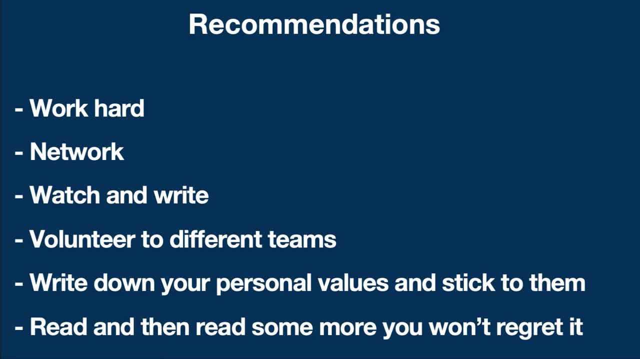 and you'd find yourself more motivated, more inspired to work hard because it's something that you enjoy. Network: like I said before, try and meet people, try and get your name out there, try and get contacts because, at the end of the day, it does help when you know people. 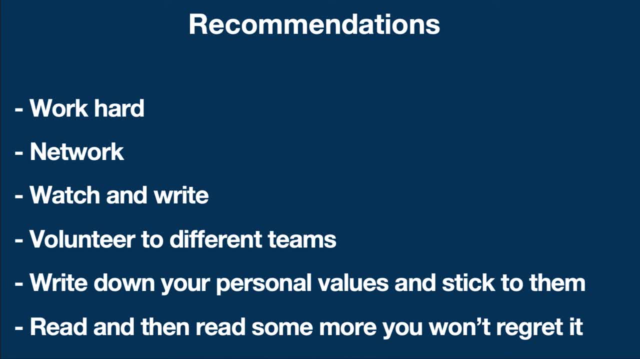 When you get your name out there and people talk, it's a very small world. So try and network as much as you can, try and travel to different places, try and meet different people, contact different people And you never know, one of the contacts may end up being: 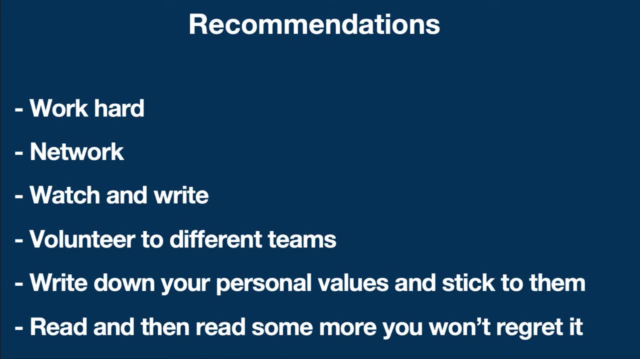 you know, getting an opportunity, getting a job, which is good, which is important. Watch and write. So watch a lot of videos online in terms of tactics, in terms of interviews, in terms of, um you know, press conferences. 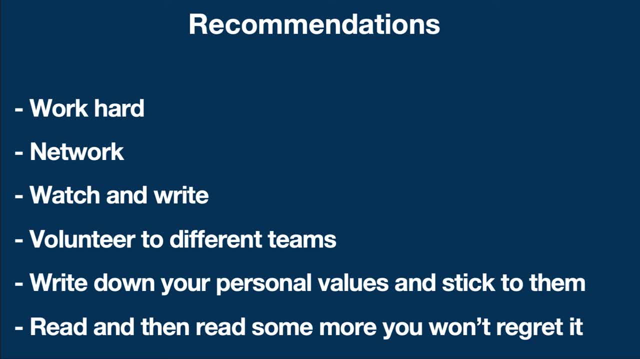 presentations on football and analysis. There's a lot of content out there that you can watch and learn. Make sure you write things down. you make notes just find it easier when I write things down when I'm reading or watching something or a lecture or presentation. 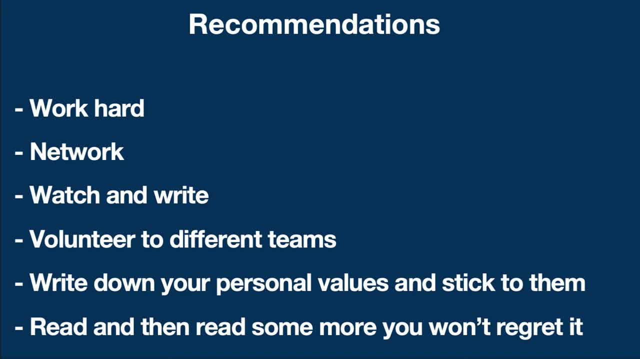 just sort of gets into my brain easier and it's my brain easier and I digest it and understand it much better. So that's important. Like I said, volunteer to different teams, volunteer yourself, get yourself out there on social media, contact different people. 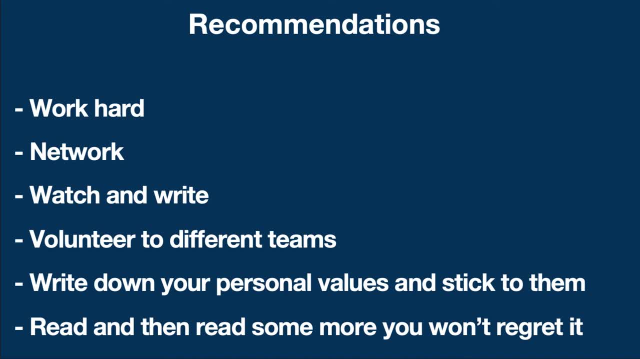 write down your personal values and try and stick them to sit down in a minute, for you know, for for a couple of an hour or two, and just really think deeply in terms of what you actually believe in. What are your humanistic values? 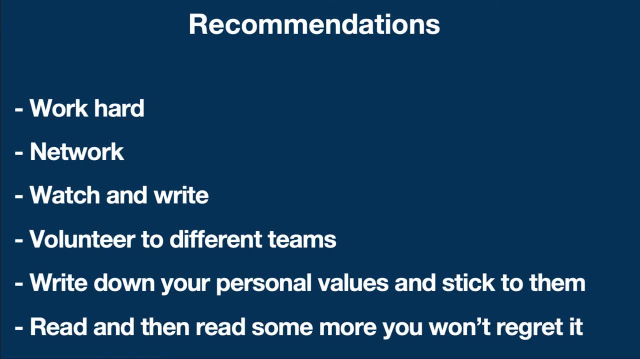 What do you believe in, What do you consider yourself as, What type of person, What's your philosophy on life and how do you think? and write them down And be very truthful and honest to yourself, whatever it may be, and then just try and stick to them. 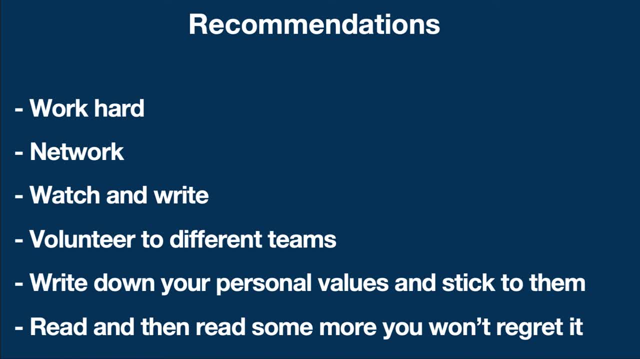 Principles. whenever you have to make hard decisions, whenever you're backing back against the wall, just stick to them, the values, and I'm sure it'll help you to get you along in life. and then read, read, try and read as much as you can. 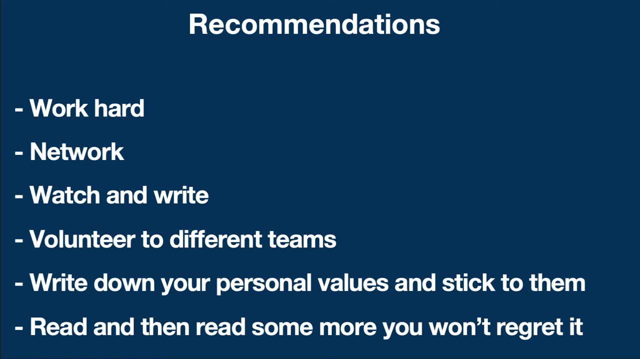 It's so important to read, train your brain again, find the subject that you're interested, because obviously that'll make it much easier. And once you find your subject, just just keep reading and reading and reading and just learn so much. So I really recommend that you read and you and you learn as much as you can. 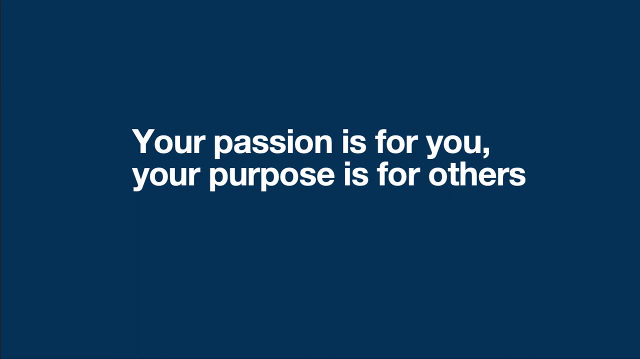 Just finishing off with a with a quote that I like, read the other day: Your passion is for you, Your purpose is for others. Like I said before, comes back to the beginning of the presentation, Make sure you find what your passion is. 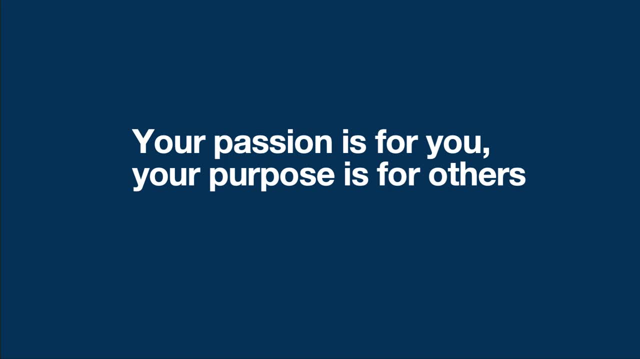 which is for you, which is going to drive you, which is going to motivate you, And then your purpose in life is for others. It's always important to help other people, to inspire other people. I think you get a lot of satisfaction and value to that when you're helping other people. 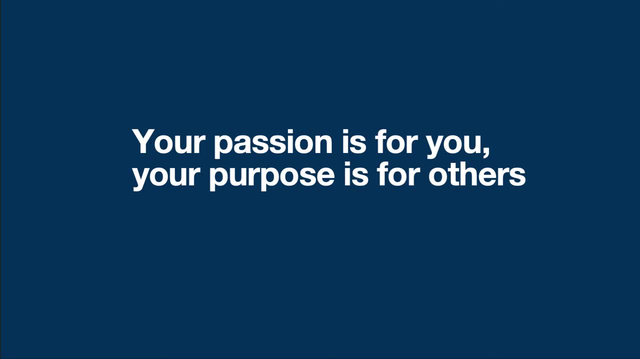 I think it's what life's about. We're here to help one another and especially help the future Yep. So I hope you've enjoyed it. If you have any questions, Chris can pass you my email. It's no problem at all. 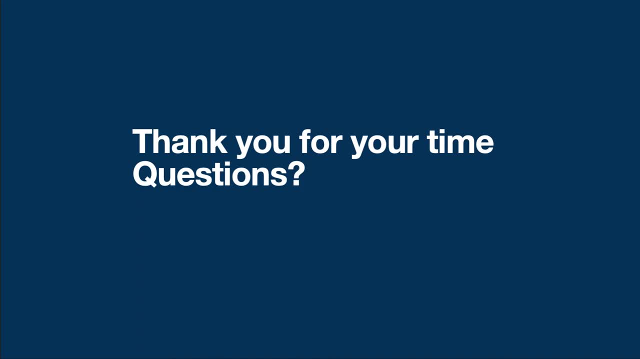 You can contact me more than happy to help out, But I hope this presentation try to keep it short and brief as possible Without boring you. Yeah, I hope you've enjoyed it. I hope you took at least something from it which you can use in your in your future. 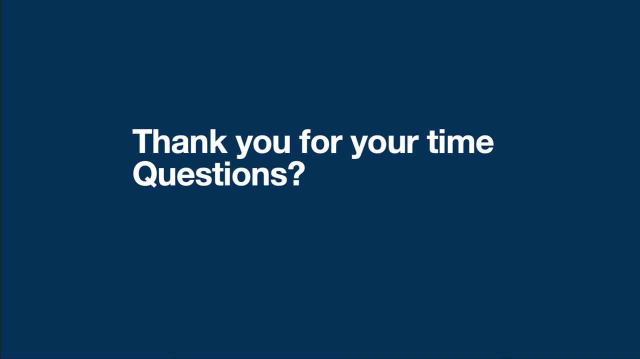 Whatever career path you may choose, just try and take them. principles I spoke about with you. I'm sure, I'm sure they really benefit you and help you. But yeah, obviously, like I said, in terms of the questions, if you do have any questions. 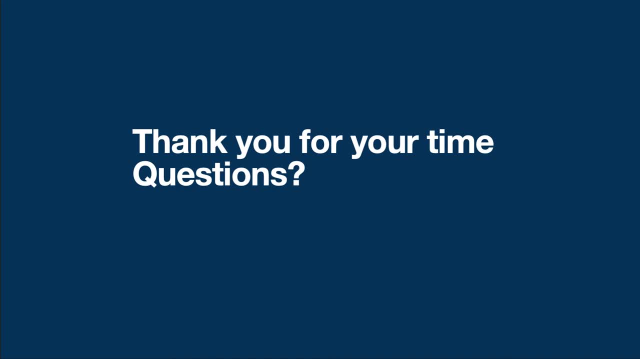 you can contact me, Chris. Chris, your lecturer can pass my information, No problem at all. Feel free to drop me an email and do my best to reply and respond. And again, yeah, thanks for your time. Thank you for listening. Yeah, I wish you all the best. 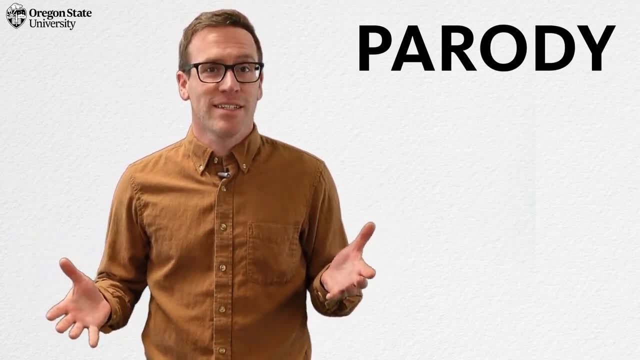 What is a parody? Well, a good definition is that a parody is a creative work that is created in order to imitate, comment on, critique and or mock its subject. It's usually, but not always, meant to be funny, at least a little bit, And the subject of a parody is often another work of art.